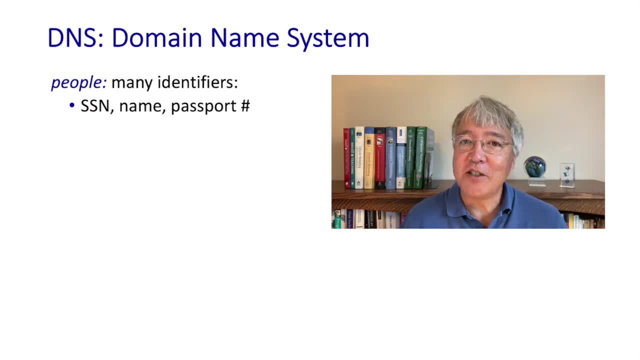 the DNS is all about names and identifiers And, as a person, I have many identifiers associated with me. I have my name, my social security number, I've got my passport ID, I've got my UMass employee ID associated with me, And we've already seen that internet hosts also have at least two. 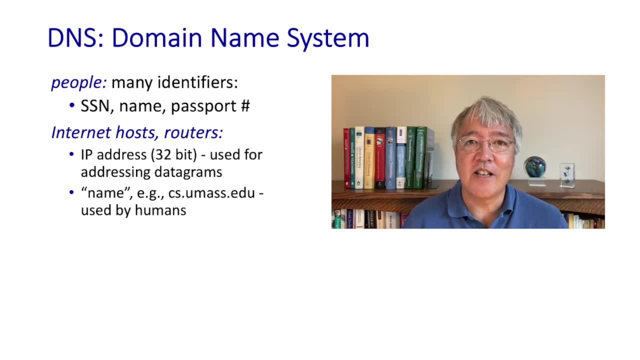 identifiers associated with them. They've got a name like gaiiacsumassedu. They've got a name like gaiiacsumassedu. They've got a name like gaiiacsumassedu. They've got an IP address like 128.119.40.186.. As we'll see, the role of the DNS is to provide. 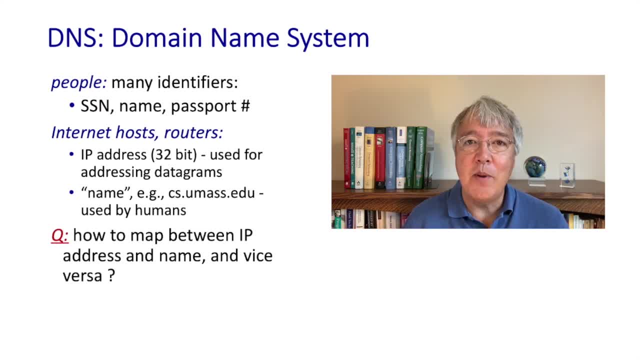 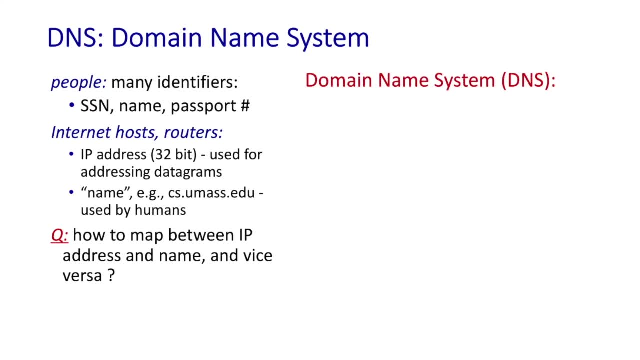 translation between names and services and IP addresses. The domain name system, the DNS, is a distributed database. The contents of this database are the records containing information about the translation among the host names, services and IP addresses. The DNS itself is a hierarchy of servers spread around the internet. 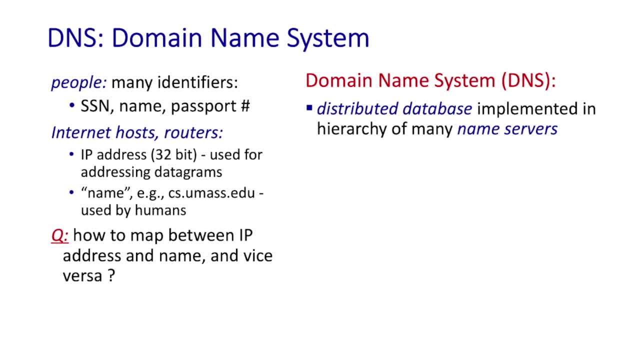 services that communicate with each other to provide this name translation service. It's important to note that the DNS is implemented as an application layer service. It's implemented by servers that sit at the network edge rather than at routers and switches inside the network, And this reflects an internet design philosophy of keeping the network core simple and putting 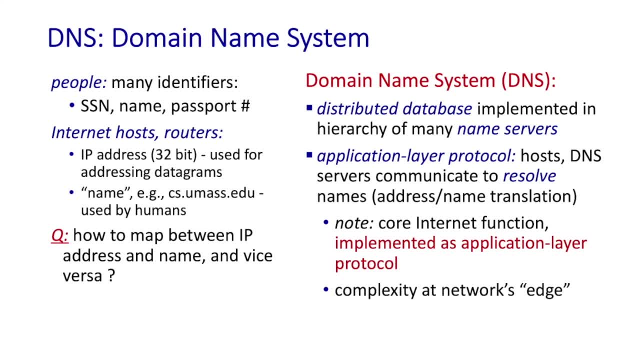 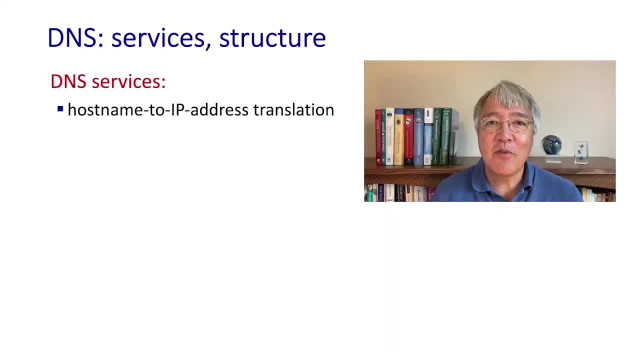 complexity at the network's edge. We'll see this design philosophy coming up again and again as we dive down into the transport and the network. And as we look at the network, we'll see that the DNS provides a number of different functions. The one we've heard about the most is this IP address. 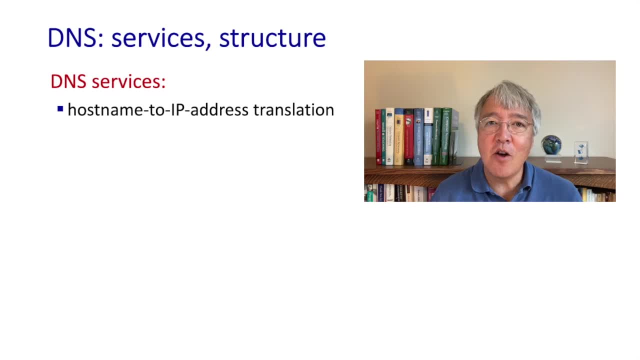 to host name translation service, But it provides a number of other important services as well. It provides an aliasing function that is, translating from externally facing names like mailcsumassedu to some internal host name. that's much more complicated than that. It also 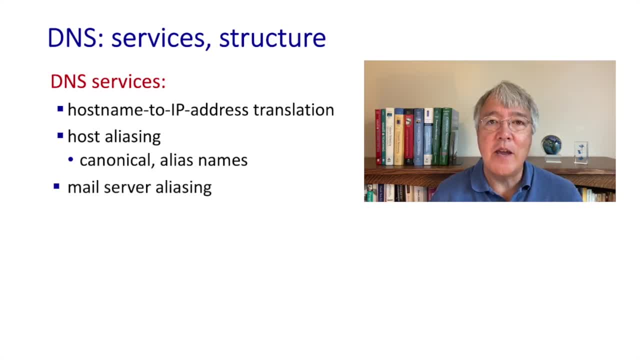 provides service resolution, for example, returning the IP address to the host name translation service. You'll notice that the DNS uses the code DNS to anchor to an IP address of a mail server associated with a domain and finally performs load balancing. There may be a number of IP addresses that are. 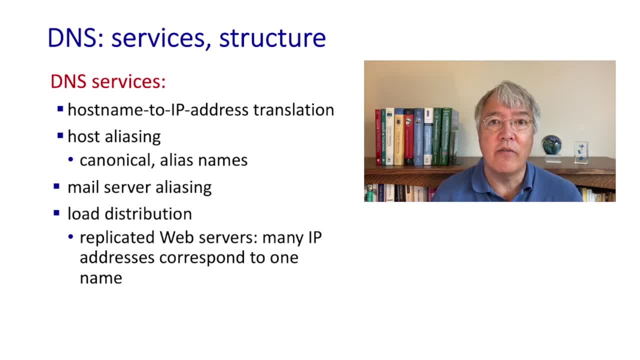 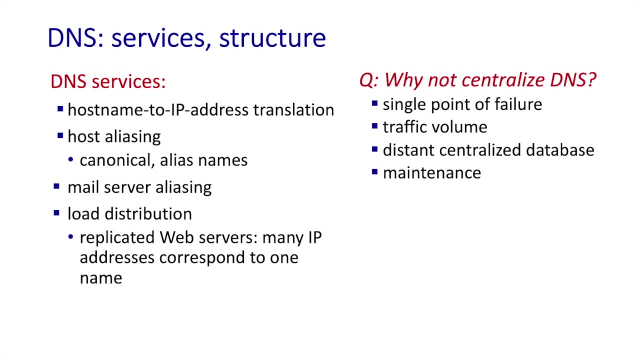 able to perform a requested service, for instance, a web server, for example, And the DNS will rotate among those possible IP addresses, returning one of those as the primary service and thus performing a kind of load balancing function, Given the DNS takes a distributed 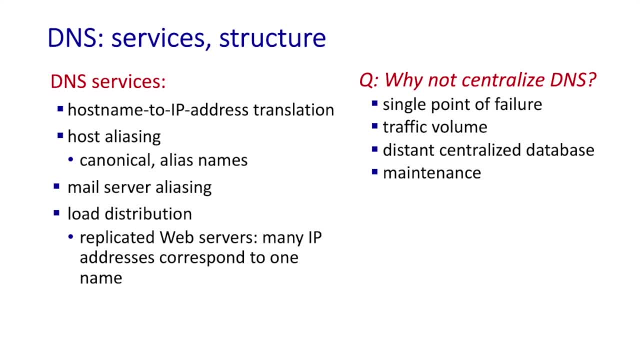 decentralized approach. you might ask yourself, why didn't the API exists? And, of course, if the API exists, then they couldn't effectively change its spectrum. designers of the DNS take a more centralized approach, and there are several considerations here. A centralized approach represents a single point of failure and we've seen that the DNS is. 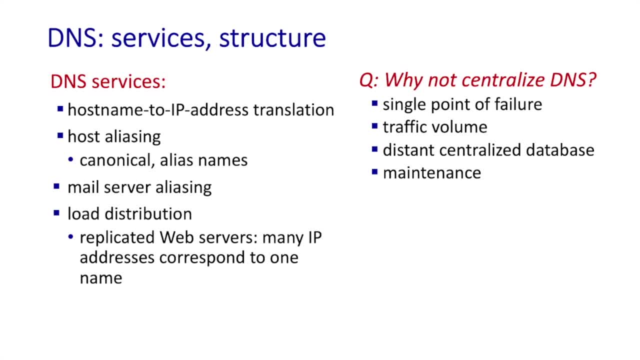 critical infrastructure. Given the loads on the DNS, a centralized approach would create a tremendous concentration of traffic And, given how important performance is- remember milliseconds count when resolving a DNS query- placing it at one location would necessarily mean long RTT delays to some places on the planet. And this is all to say that a centralized approach simply doesn't. 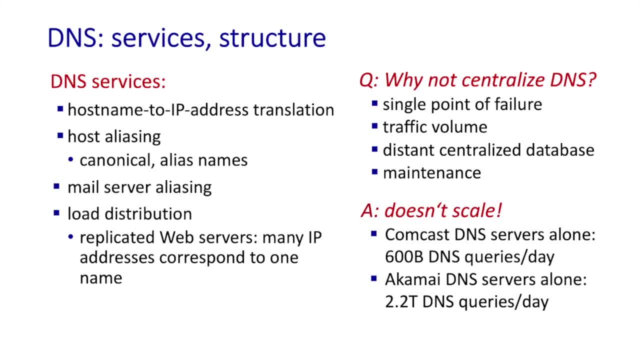 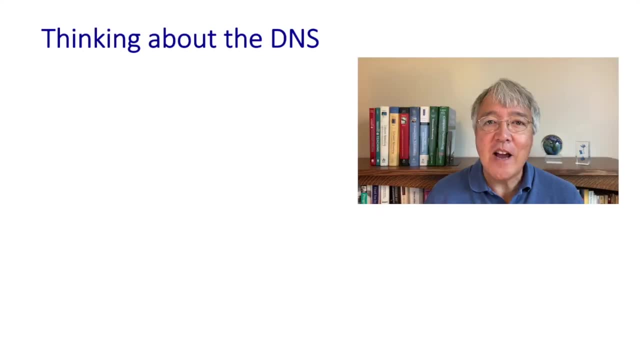 scale With trillions of queries a day. Akamai alone handles more than a trillion DNS requests a day. A single centralized service doesn't have the computational capabilities, the resiliency or the performance that one can get with a decentralized approach Well before diving. 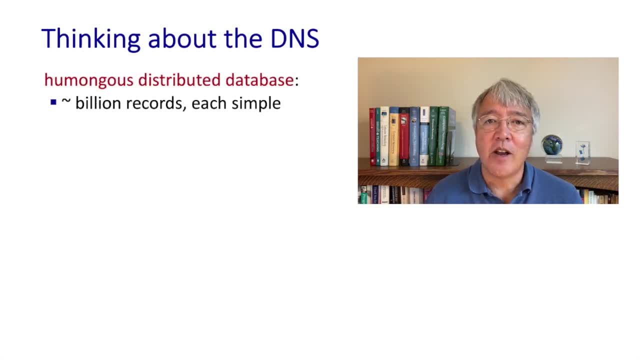 into the technical details of the DNS. let's summarize here in terms of how to just even think about this, The DNS, So you can think about it as a highly distributed, high scale, high performance, distributed database. That's a tough problem, but at least, as we'll see, the records are relatively 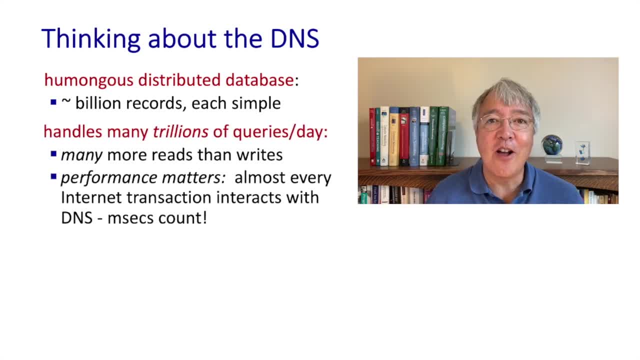 simple And you want to think about it in terms of performance and scale. also, It needs to be able to handle literally trillions of requests- mostly reads- that come in every day, and it has to do so with really high performance. Milliseconds are going to count, And then organizationally, it's. 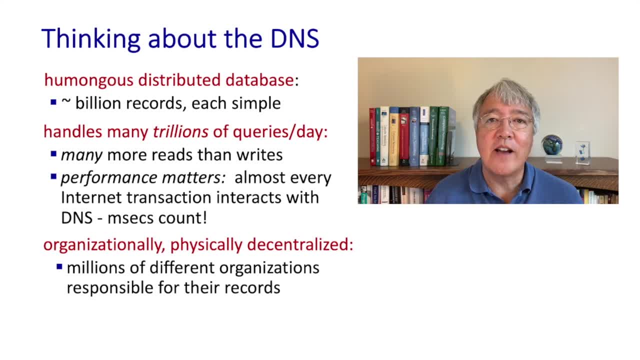 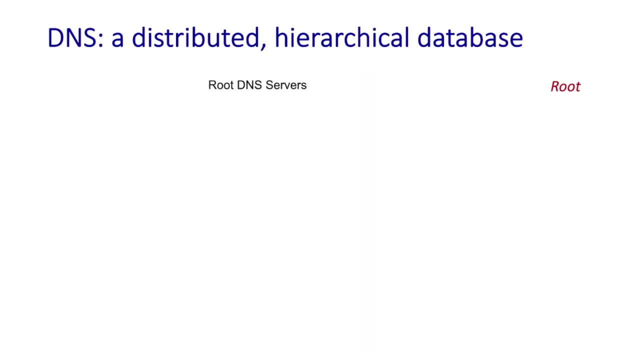 also highly decentralized. There are literally hundreds of thousands of organizations that are going to be responsible for their pieces, their records, within this distributed database. Is this an easy problem? Not really. Well, we said that the DNS is a distributed hierarchical database. 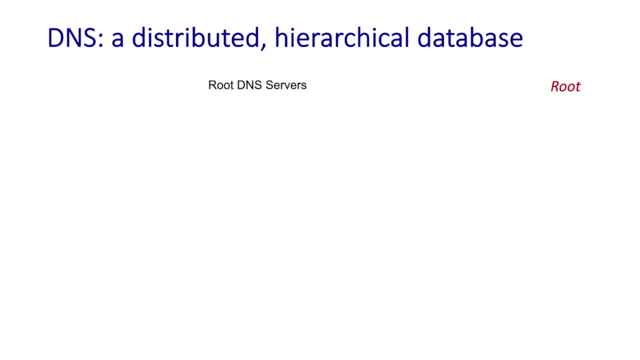 So let's take a high level. look at this hierarchy, The root of this tree. we have the root DNS servers. The next layer: we have the DNS servers that are responsible for all of the data that's available for all of the com or edu or net domain names. These are known as the top level. 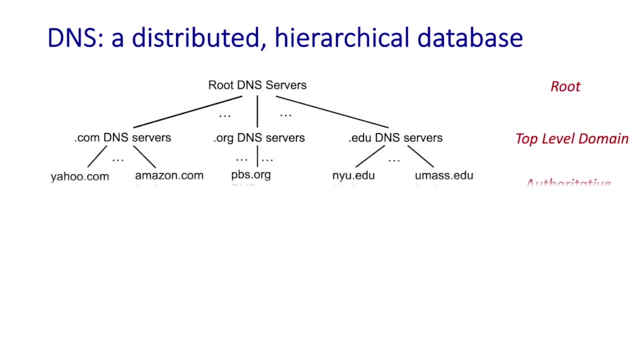 domain or TLD servers. And then we have the authoritative name servers. These are the servers that have the ultimate responsibility for resolving names within their domain, For example, for all of umassedu, all of nyuedu or all of pbsorg. Now, if a client 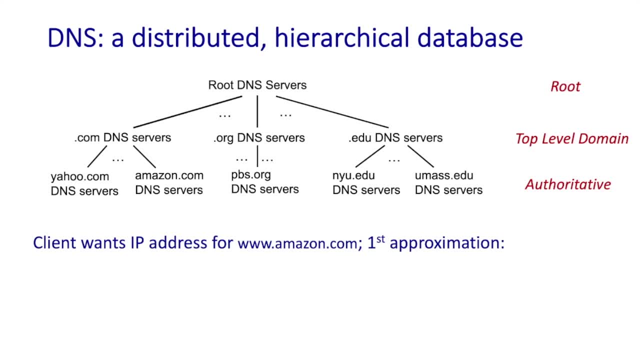 wants to resolve an address, say for wwwamazoncom. here's the basic approach. Client could first contact a root DNS server to get the name of the TLD server for all of the coms. The client then contacts the TLD server to get the name of the authoritative name. 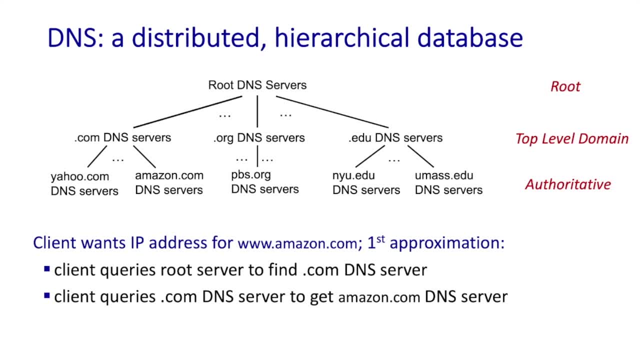 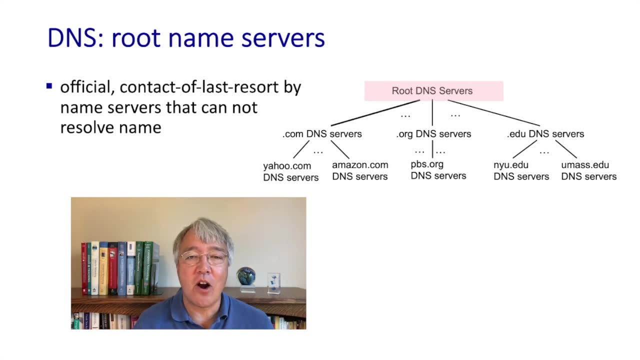 server for amazoncom. And then, finally, the client contacts the authoritative name server for amazoncom to get the IP address of wwwamazoncom. Well, since we like to study things top down, let's start at the top. Let's start at the top of the DNS hierarchy, and that's with the root servers. 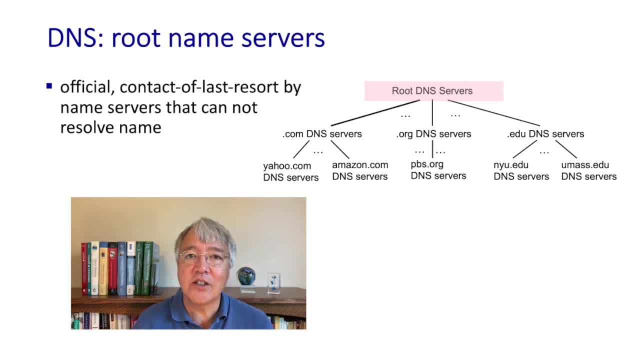 The root servers are a place to go when a server is not actually able to resolve a name. You can think of it almost like a contact of last resort, And in fact it's not really a contact of last resort because it's not going to actually provide that translation service, but it's a place to go. 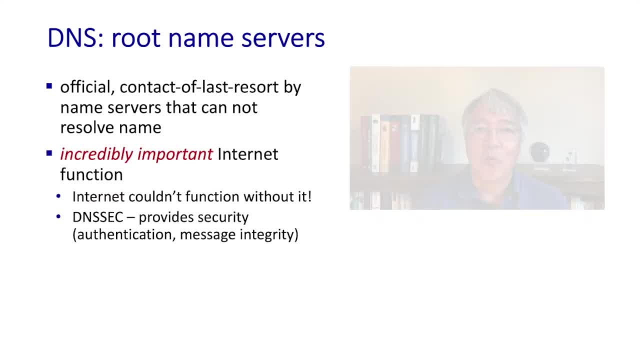 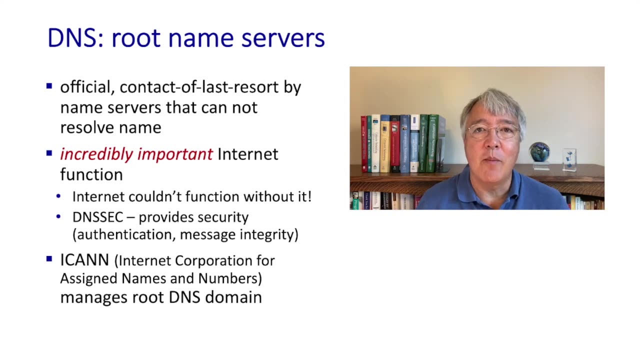 to get translation started. Well, this is obviously an incredibly important function for the internet, almost like the central nervous system of the internet, And, as such, security is going to be very important. Now, the root servers and much of the infrastructure associated with them is the responsibility of ICANN, the Internet Corporation. 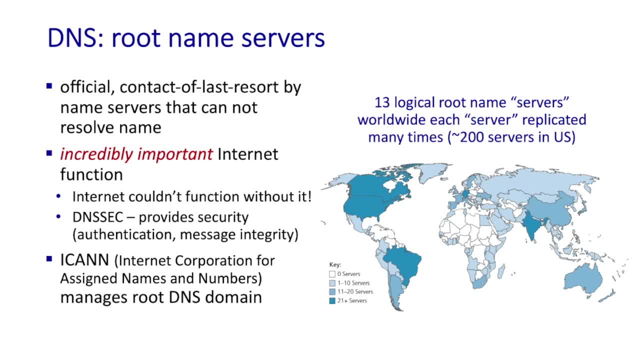 for Assigned Names and Numbers. There are 13 logical root servers around the world, but each of these logical root servers are themselves actually replicated, So corresponding to these 13 logical servers are actually close to 1000 physical servers around the world. There are more. 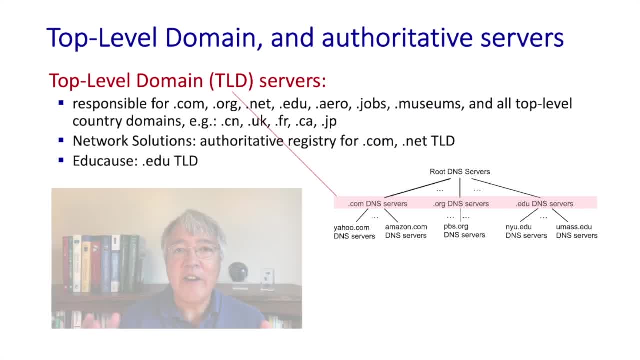 physical root servers in the US. Moving down a level from the root domain, we find the TLD, the top level domain, And each of the servers in the top level domain is responsible for resolving one of the addresses that have an ending like com, edu, net or org- The associations that 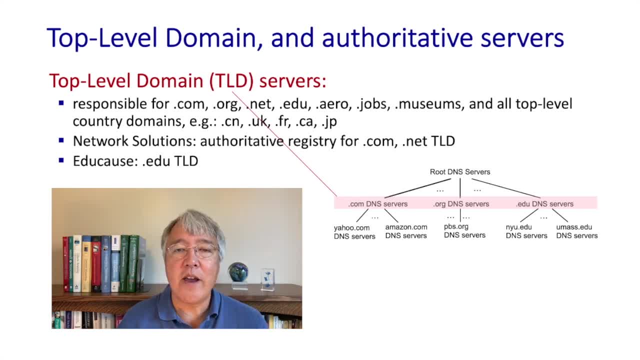 are responsible for managing these TLD domains are known as internet registries. These internet registries are also the place that you'd go. If you want to know more about the TLD domain, you can go to the Internet Registries website. 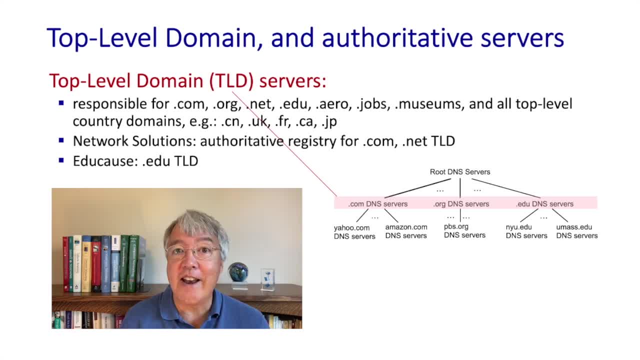 If you want to know more about the TLD domain, you can go to the Internet Registries website. If you want to know more about the TLD domain, you can go to the Internet Registries website. If you want to register a new com, edu or net name, the authoritative name servers are responsible for. 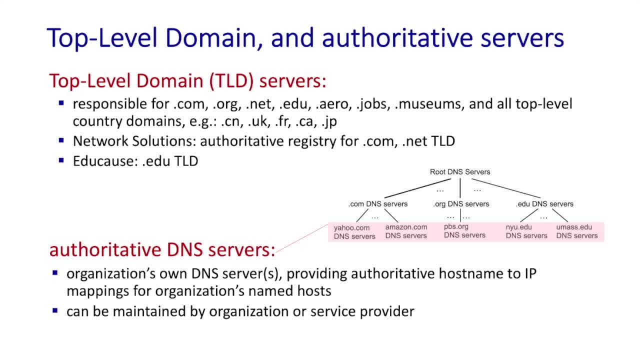 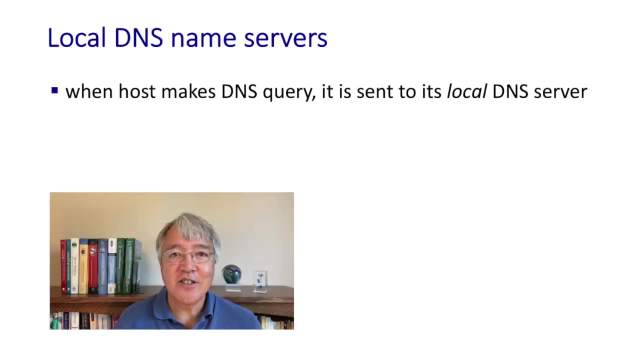 resolving names within an organization, And such a server is authoritative in the sense that, as the saying goes, the buck stops here. This is the DNS server that has authority over the organization's names, And what this server says goes. And lastly, there are the local DNS servers. Every host on the internet has an associated local DNS. 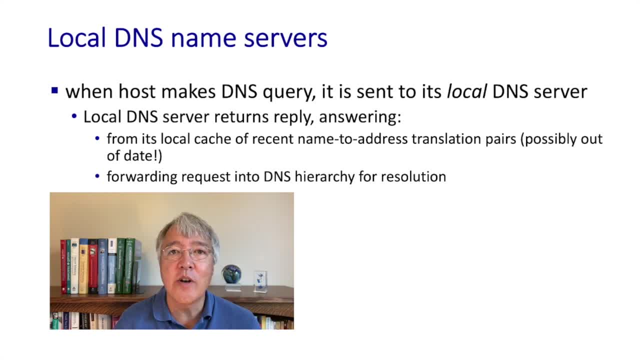 server And this is the name server that a host is going to contact when it wants to resolve a name. The local DNS name server is then going to respond immediately to the requesting host if it has that name-to-address translation pair cached locally. Otherwise it's going. 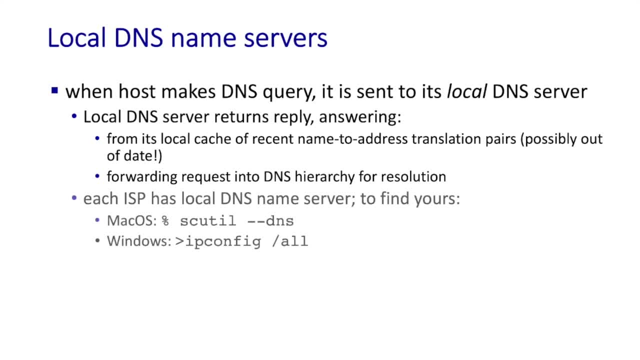 to start the resolution process. If you're interested in finding out the host name of your local DNS server, you can type in one of these two commands into your computer. Under macOS type, in scutil, __dns or under Windows, ipconfig. all Each of these commands displays the name. 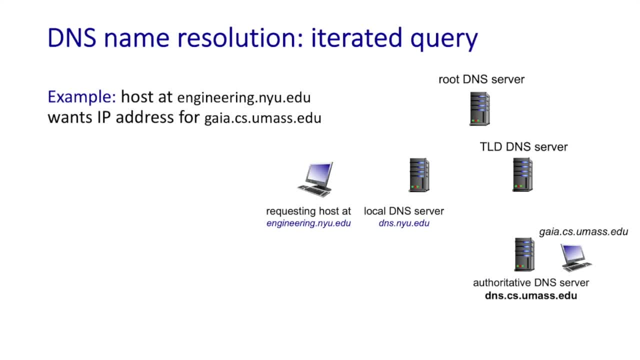 of your local DNS server. Now let's take a look at an example of DNS name resolution in action. Suppose the requesting host is at engineeringnyuedu and it's going to make a request to resolve the name gaiacsumassedu. Well, here's how this unfolds: The host at engineeringnyuedu. 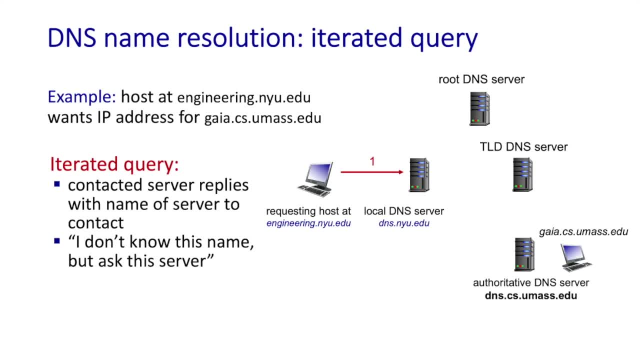 first sends a DNS query message to the local NYU DNS server, let's say dnsnyedu. The query message contains the host name, to be translated gaiacsumassedu. Now it's the job of this local NYU DNS server to resolve this name. It begins by forwarding a query message to a root DNS server. 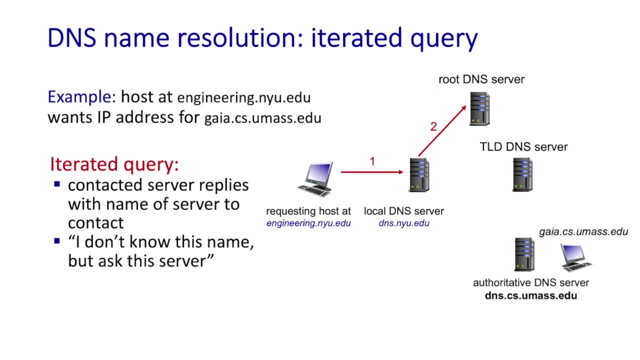 The root DNS server takes note of the edu suffix and returns to the local DNS server a list of IP addresses of TLD servers- top-level domain servers responsible for edu. The local NYU DNS server then resends the query message to one of these TLD servers. The TLD server takes note of. 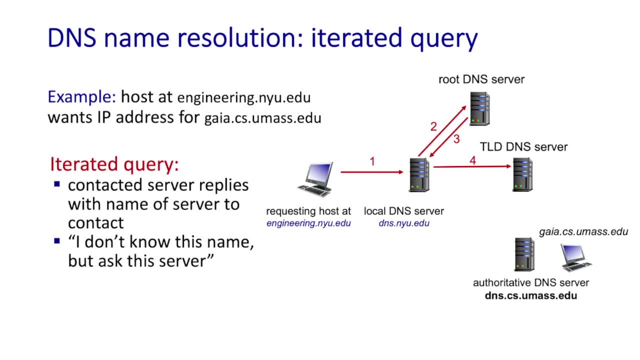 the umassedu suffix and responds with the IP address of the authoritative DNS server for the University of Massachusetts, dnsumassedu. Finally, NYU's local DNS server resends the query message again to dnsumassedu and UMass's authoritative name server responds with the IP. 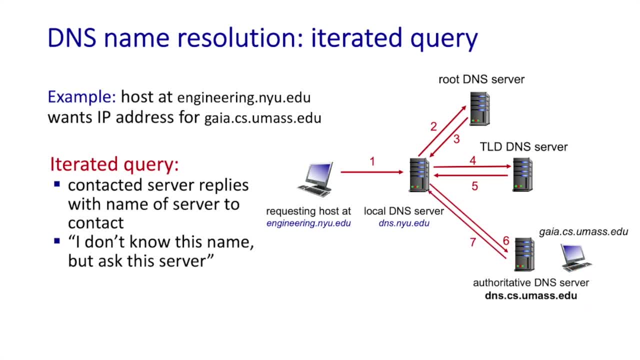 address of gaiacsumassedu. In order to get the mapping for one host name, eight DNS messages were sent: four query messages and four reply messages. We'll see soon how DNS caching can reduce this query traffic. The type of querying that we've seen in this example is known as an iterated query. 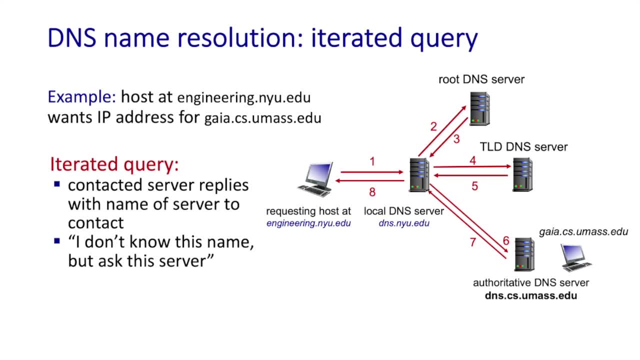 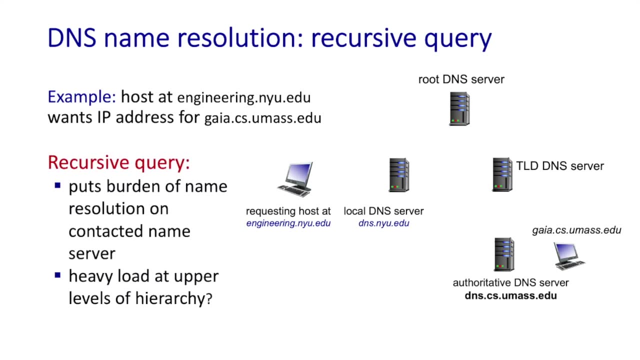 because the local DNS server at NYU is iteratively querying a sequence of servers until finally the gaiacsumassedu name is finally resolved. A second form of query resolution is known as recursive query resolution. In recursive query resolution, rather than responding to a request, 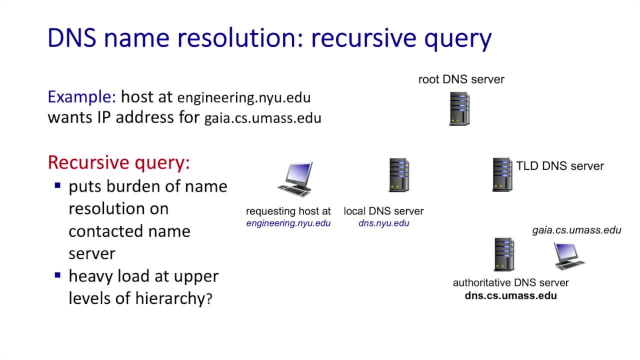 with a I don't know, but here's who to try. next type of response that we saw with iterative queries: the name server takes it upon itself to resolve the query. The name server takes it upon itself to resolve the query and return a definitive reply. In this example here, which shows a cascade of 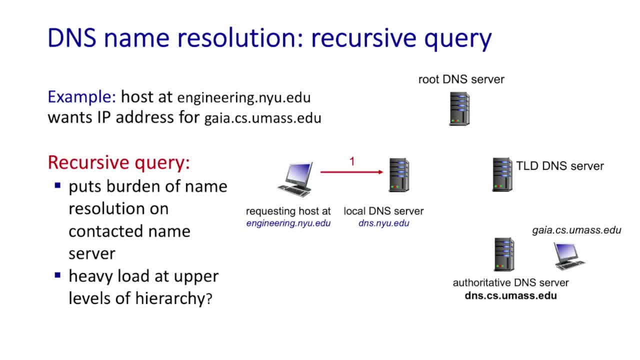 recursive queries. the local DNS server at NYU again queries the root server. In this recursive case, however, the root server queries the TLD server. who queries the UMass authoritative name server? who replies to the TLD server? who replies to the root server? who replies to the local DNS? 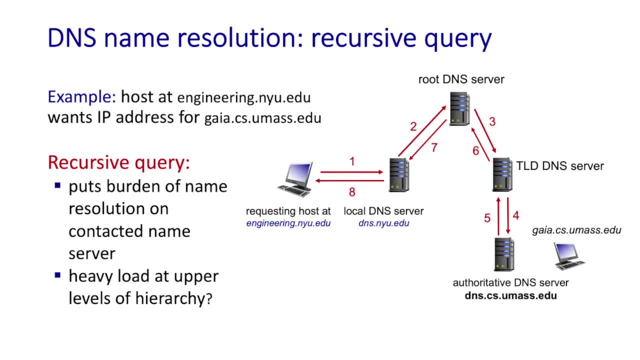 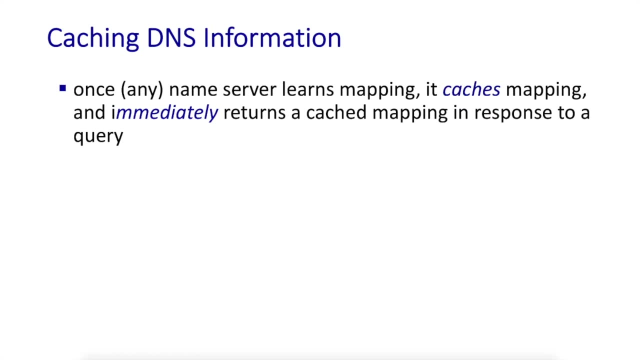 server at NYU who replies to the querying host. Because this form of recursive querying puts the burden on the servers at the upper level of the hierarchy, it's not often used in practice, and instead iterative querying is adopted by the local DNS server. Now we've seen that a lot of work can be involved in obtaining the DNS record. 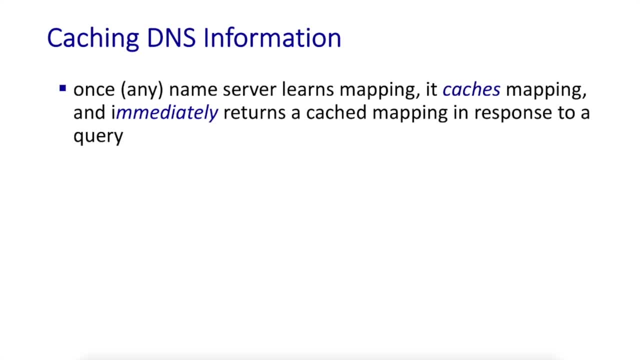 for a name-to-address translation pair. so it'd be great to somehow leverage that work and remember, that's to say cache that record locally for some time in case another request comes in for the same record. So once a DNS server learns a mapping, it's going to cache that mapping for. 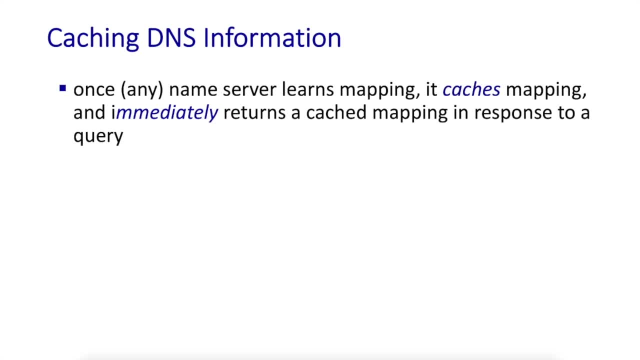 some amount of time. If a future request comes in for that mapping, it can immediately return the cached reply in response to the query. So we see that caching improves response time and it takes load off the DNS infrastructure- a double win. Cached entries will eventually. 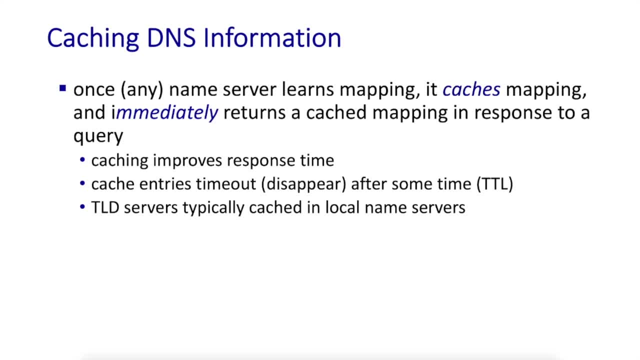 time out and disappear from the cache after some amount of time- the time to live. Note, however, that it's possible that if a DNS record changes, the cached entries will then be out of date. However, the DNS doesn't worry about stale and out-of-date cached entries. They'll time out. 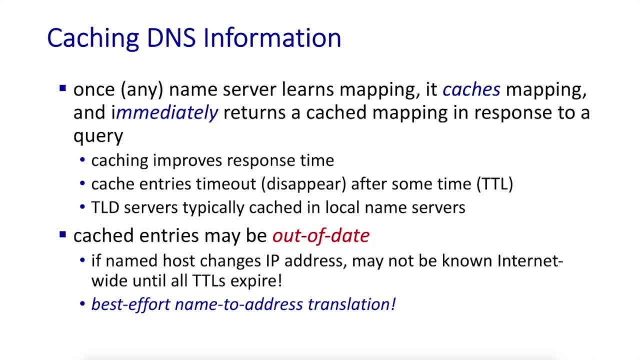 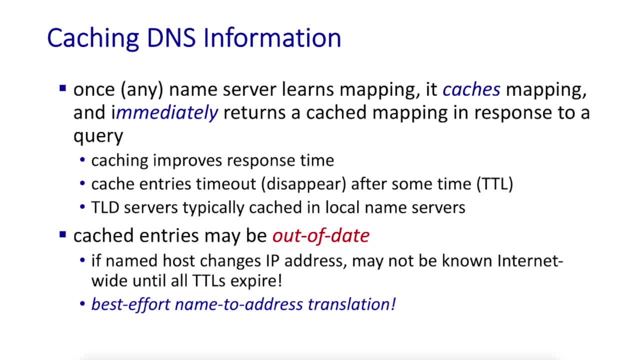 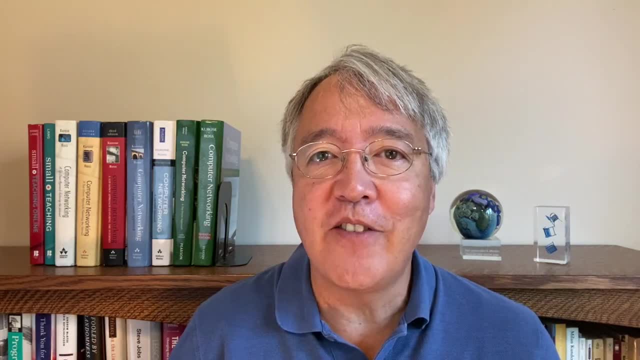 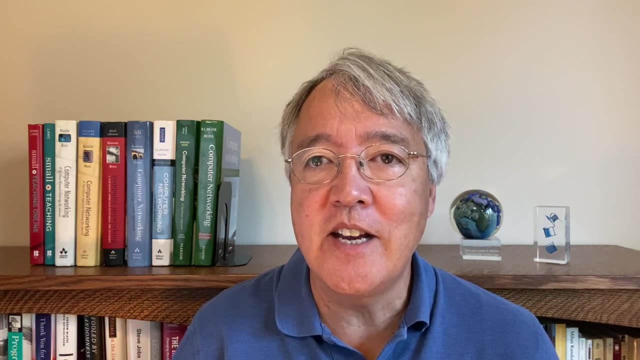 Well, that's all we want to say about the structure and the function of the DNS, but there's still two more things we want to take a look at. We want to take a look at the resource records that are inside the DNS, and we want to take a look at what DNS protocol messages look like. 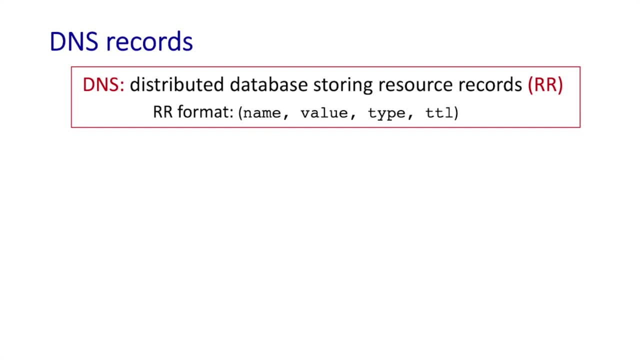 DNS database records are a four-tuple with a name, value, type and TTL or time-to-live field. There are a number of different types of DNS records, but here are four popular ones. When the type is A, that is an address record, the record contains a host name. 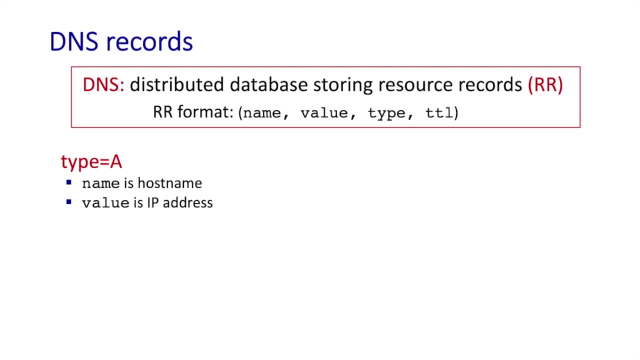 and its IP address, And this record is used for name-to-address translation. When the type is NS- a name server record, the name is a domain name, like umassedu, and the value is the host name of the authoritative name server for that domain. A CNAME record is used for name. 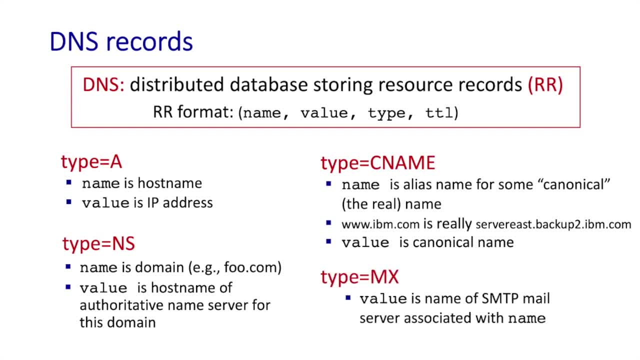 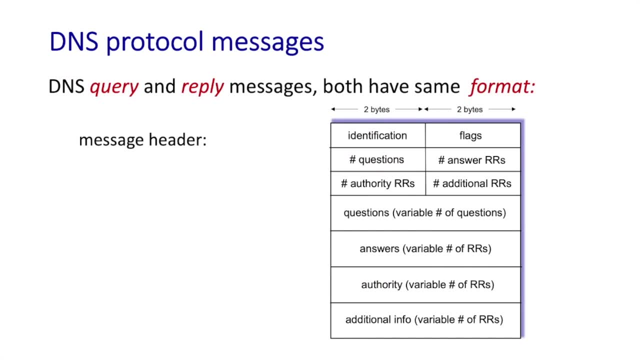 aliasing, and an MX record is used to give the name of a mail server associated with the domain. Let's next take a look at the DNS protocol message formats. Both the query and the reply message have the same format, as shown here on the right. Remember that the DNS is a query response. 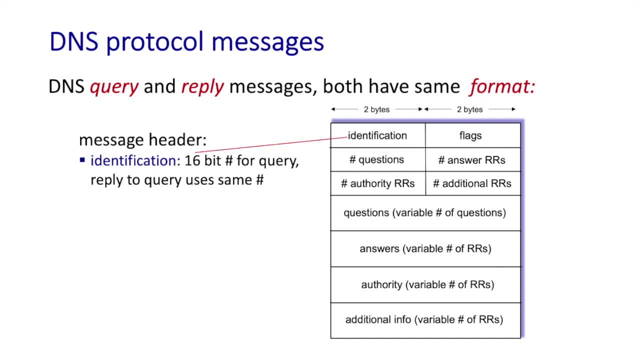 protocol. The ID field here is a 16-bit number chosen by the querier. When a response protocol response is sent in REPLY to a query, that response takes its ID value to be the same as that of the query to indicate that this is a response to that particular query. 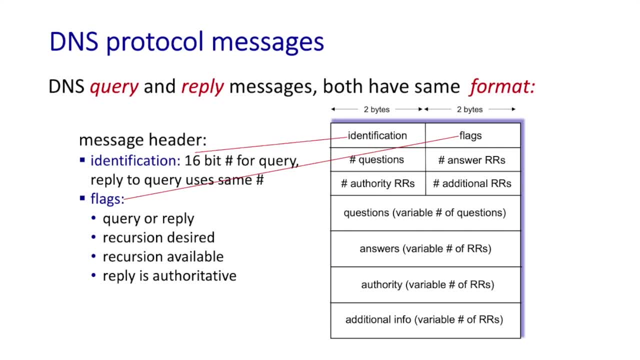 The FLAG field is used to indicate whether this is a query message or a requiry message if it's conquering aufavorable thought-豐. The next four fields are used to indicate the number of questions. 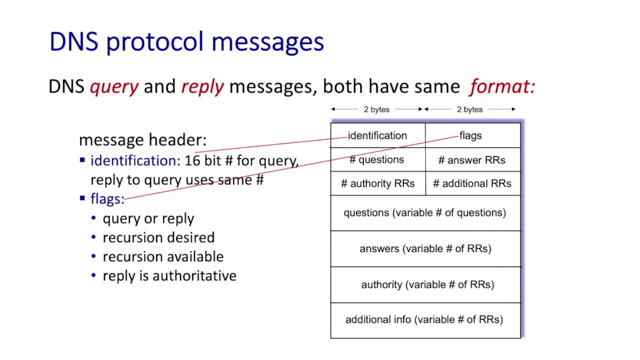 and responses in the remainder of the protocol message. Number of questions, Number of responses. a query, a question, say to resolve a host name to an IP address, the host name would go in this field here, In the case of a reply to such a query, a resource record of type. 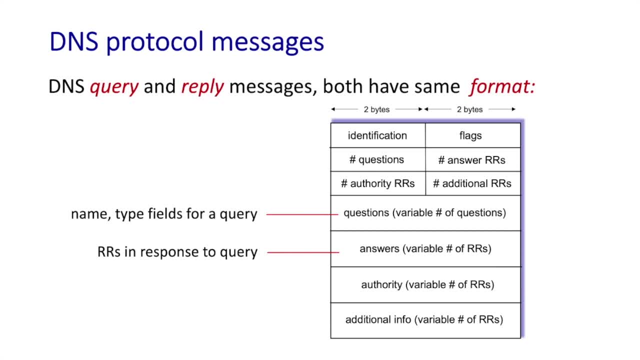 A remember containing the name and the IP address of a host would be inserted in this field here. RFC 1035 defines all of these fields and resource records as well. To help put together the pieces of some of what we've learned about the DNS, suppose, 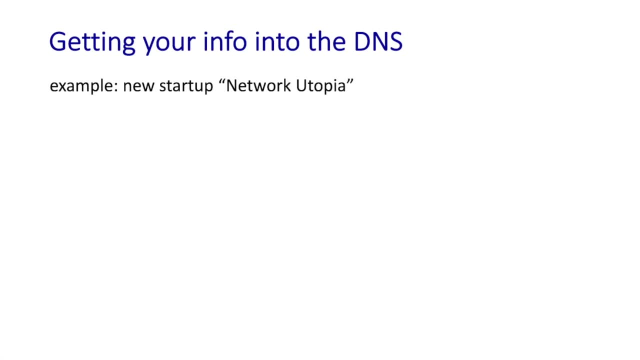 now that you create a company, it's called Network Utopia. It's got a network and you want an internet presence. You want your company services to be reachable by others on the internet at your site, Network Utopiacom. What do you need to do? Well, clearly, the 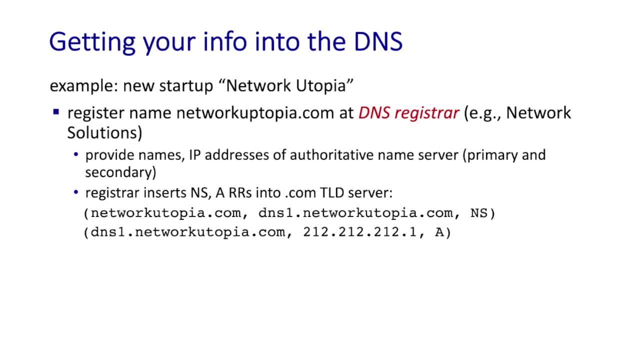 DNS is going to be involved, since, in order for users to reach your network, they'll need the IP addresses of the servers in your network. And even if the name Network Utopiacom becomes fabulously famous, no one's going to know the IP addresses of the network. 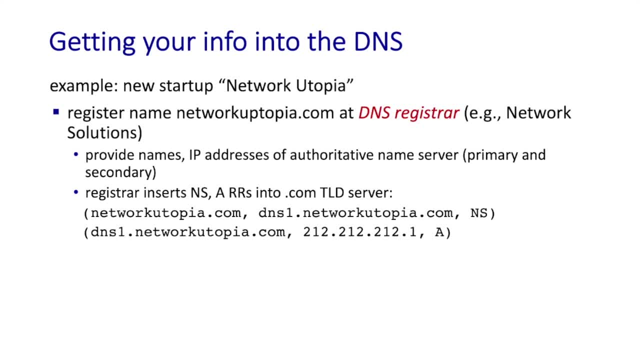 of your servers. So of course you'll need to use the DNS for that. First you register your name networkutopiacom with a DNS registrar, like Network Solutions, a company. that's a registrar that we mentioned earlier. You'll need a set of IP addresses. also We'll discuss in chapter four. 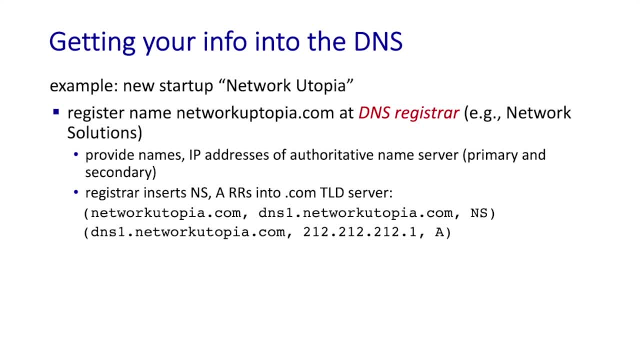 how you get those. so let's assume for now that you've got a range of IP addresses for your servers. You then need to give the name and address of your authoritative name server to the registrar. The registrar will insert your name server's name in an NS record and its IP. 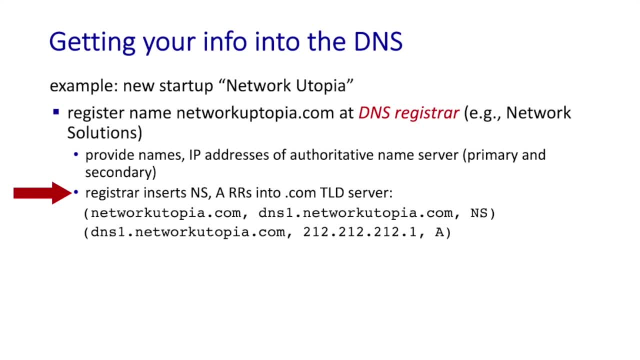 address in an A record into the global DNS database. That's all that needs to be done with the registrar. The addresses of all the other servers in your network will be provided by your authoritative name server to queriers who know the host names for those services. And lastly, 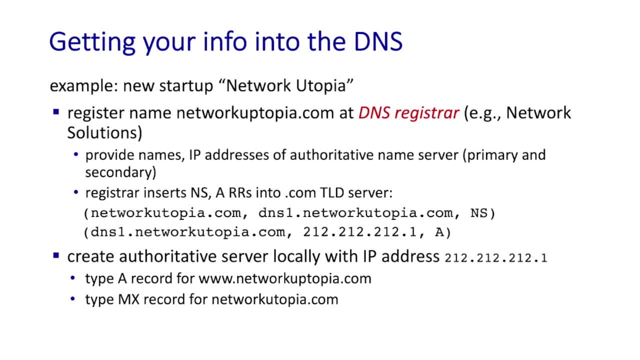 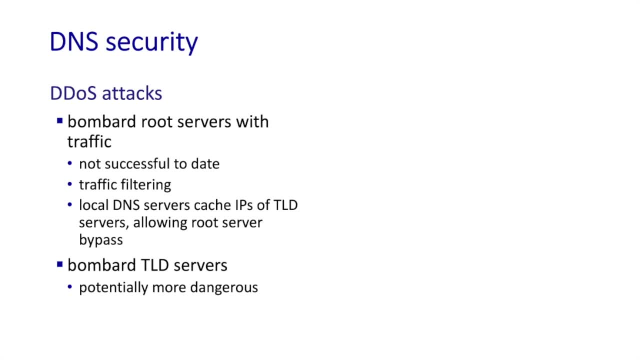 you need to bring up your authoritative name server and populate it with resource records for the servers in your network. And let's wrap up here with just a quick word about DNS security. Now that you understand what the DNS does, you can see how absolutely critical it is to the functioning of the internet If the 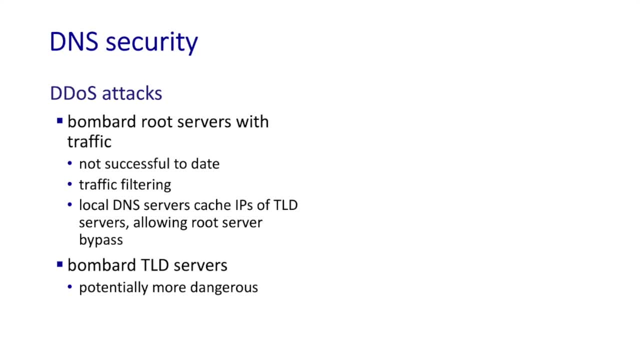 DNS stopped working. it'd be impossible to contact any host unless you knew its IP address, which means practically never, And so it's critical that the DNS be protected. The DNS is protected against denial of service attacks primarily by firewalls. The DNS also needs to ensure that. records that are in the network are protected against denial of service attacks, primarily by firewalls. The DNS also needs to ensure that records that are in the network are protected against denial of service attacks, primarily by firewalls. The DNS also needs to ensure that records that are 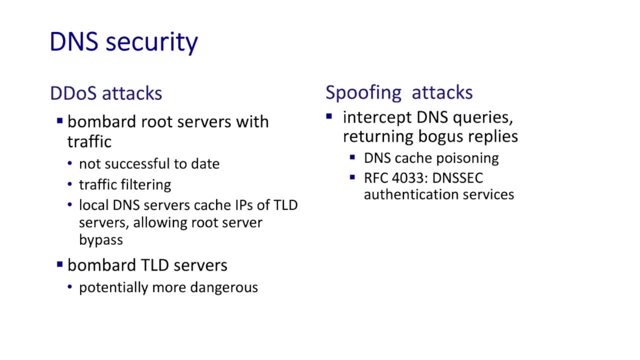 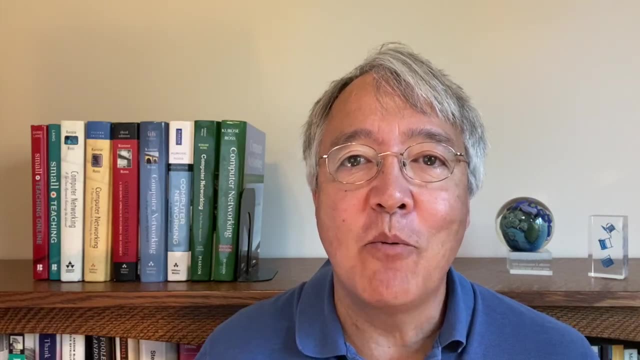 entered into the database are from authorized sources, And so authentication services will play a critical role in protecting the DNS. We'll look at authentication services when we get to chapter seven. So that wraps up our discussion of the DNS, an absolutely critical network function that has.